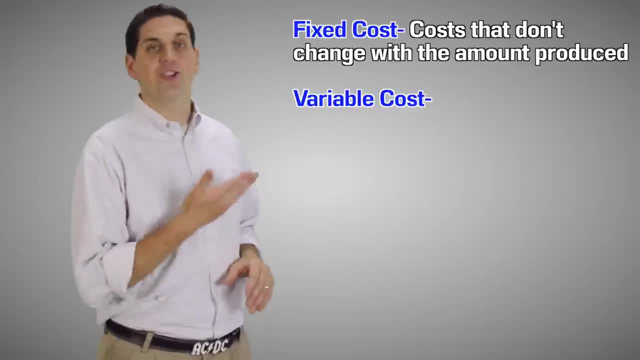 produce. It doesn't matter how many pizzas produce. It doesn't matter how many pizzas produce, You still have to pay for the oven. Another example might be the manager's salary right. You still need a manager, whether you produce one unit or a thousand units, And so the manager's 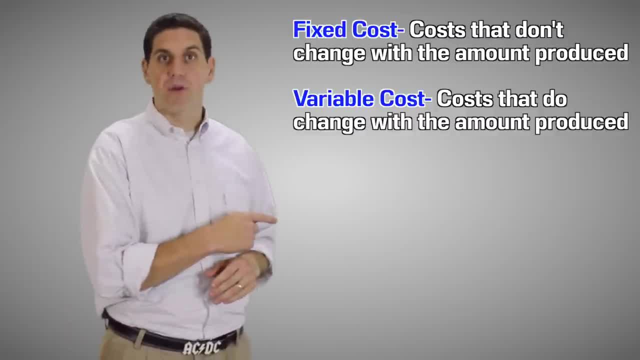 salary is a fixed cost, So variable costs do change with the amount produced. So if you produce more output you're going to need more resources. So raw materials, labor, electricity are all examples of variable resources and that's variable costs If there's only two types of. 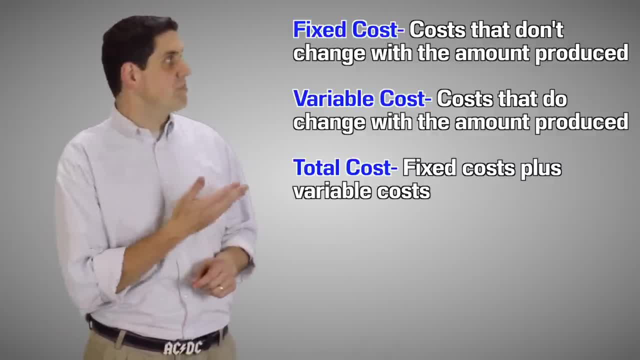 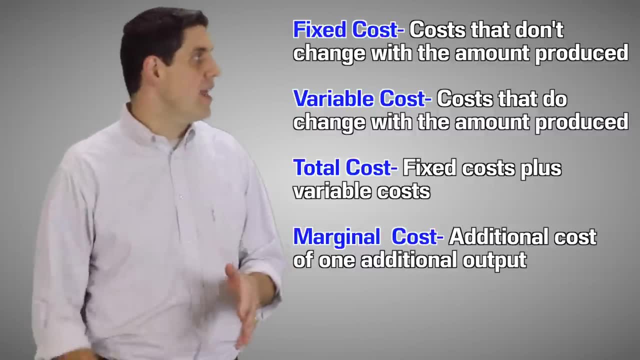 costs fixed and variable, then total costs must be fixed plus variable costs, And there's also marginal cost. Marginal cost is the additional cost of the product. So if you're a pizza company, it's the cost of producing one more output. If you're a pizza restaurant, it's the cost of 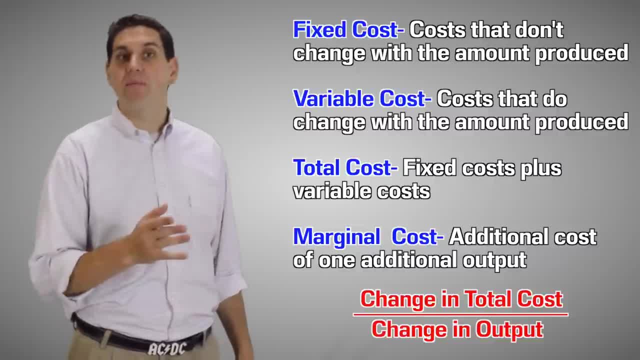 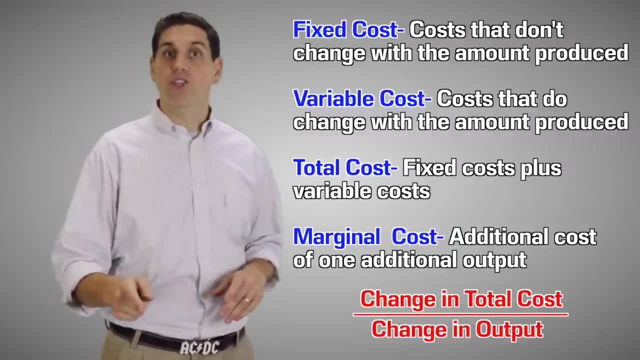 producing one additional pizza. It's the change in total cost divided by the change in output. So now you understand the total cost. There's total fixed cost, total variable cost, total cost and marginal cost. Now let's see if you can calculate them on your own Right here. 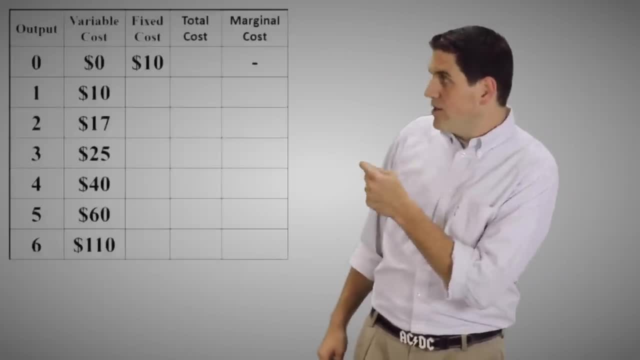 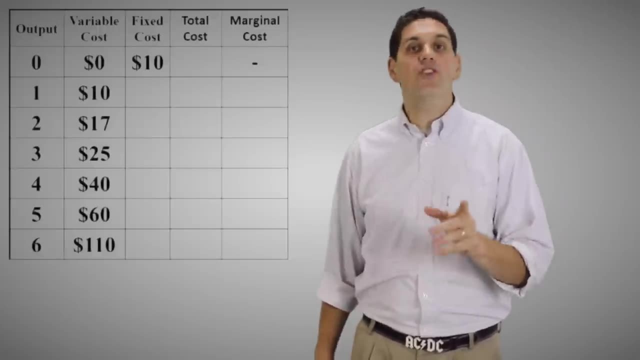 I have the cost for a given firm right. We have zero output. We got one, two, three, four, five, six units that they could produce. I've also given you the variable cost and the fixed cost producing no output. I want you to copy this chart on your piece of paper and finish off these. 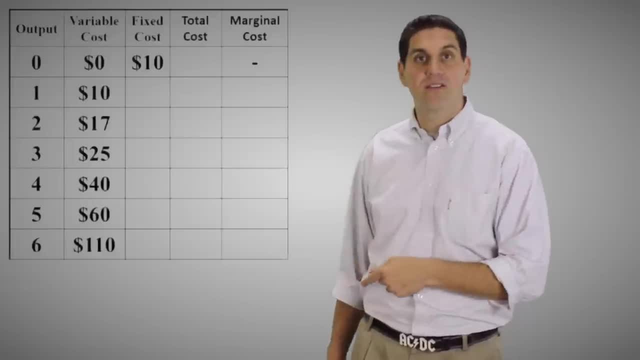 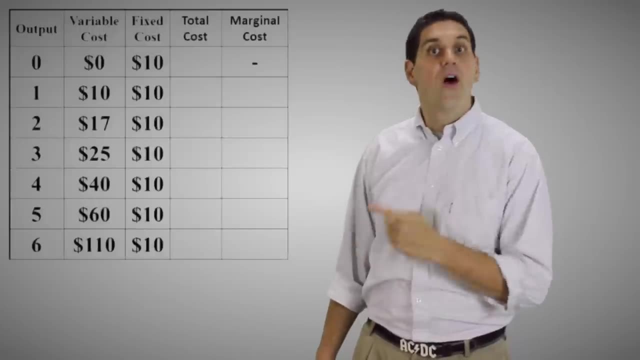 columns, Calculate the fixed cost, the total cost and the marginal cost. Pause the video and then do those calculations and I'll go over the answers. What's the fixed cost of producing one unit? Well, it's $10.. For two units, it's $10.. For three units it's $10.. Why? Because it's fixed. 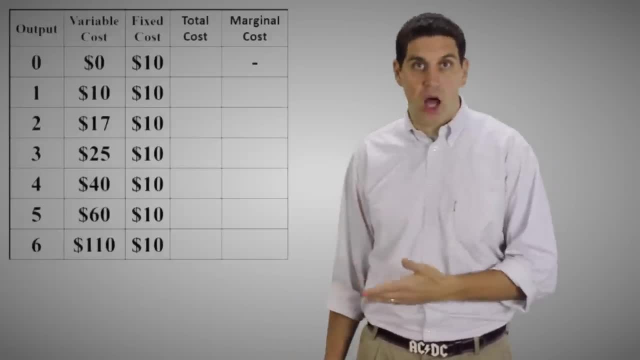 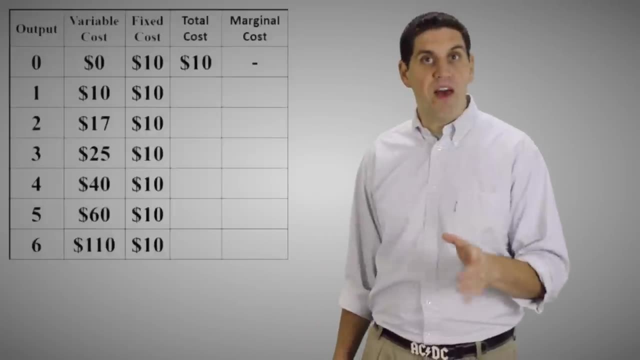 It doesn't matter how many units produced, You still pay $10 fixed cost. Total cost is the variable plus the fixed cost. So when you produce nothing you still have a total cost of $10.. Remember that's because you have to pay that fixed cost. For one unit it's $20.. For two units: 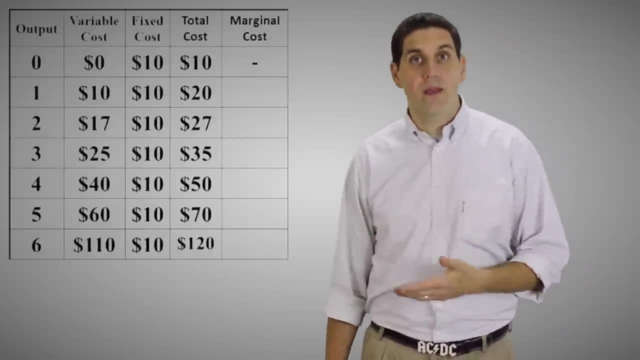 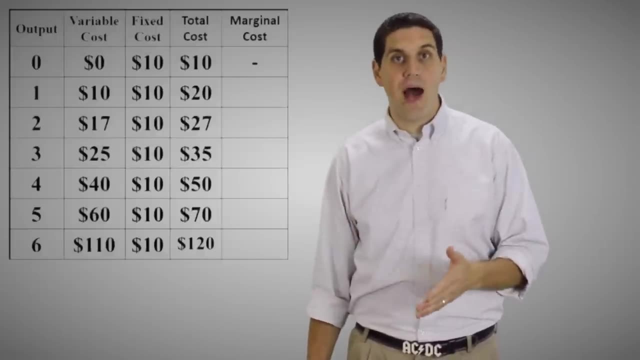 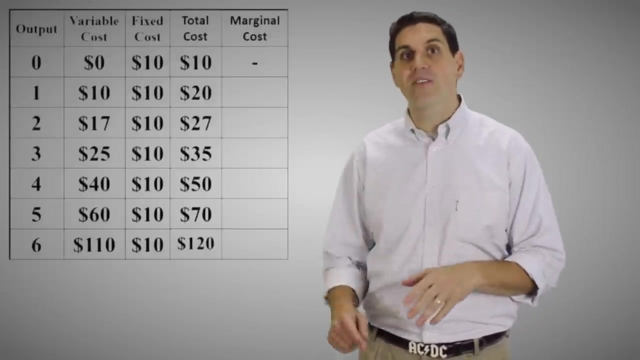 it's $27.. And it's really that simple. Variable cost plus fixed cost equals total cost. The marginal cost is the change in total cost from producing an additional output. So if the total cost of producing nothing is $10 and the total cost producing one unit is $20, the additional cost 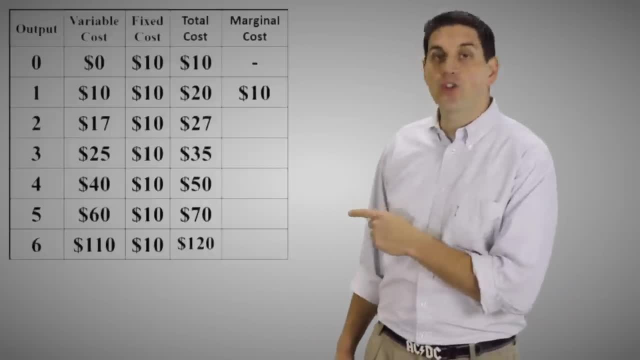 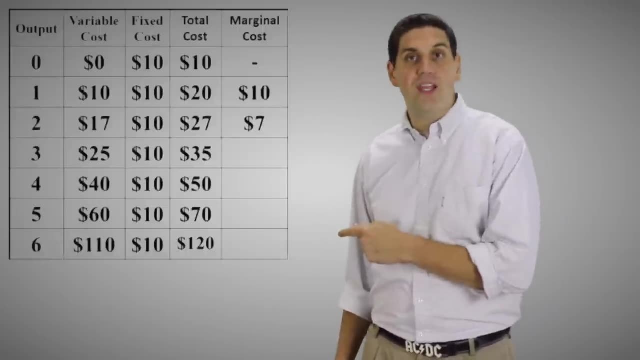 of that first unit must be $10.. Since the total cost of two units is $27,, the additional cost of that second unit must be an additional $7.. So again, the marginal cost is the change in total cost divided by the change in output. 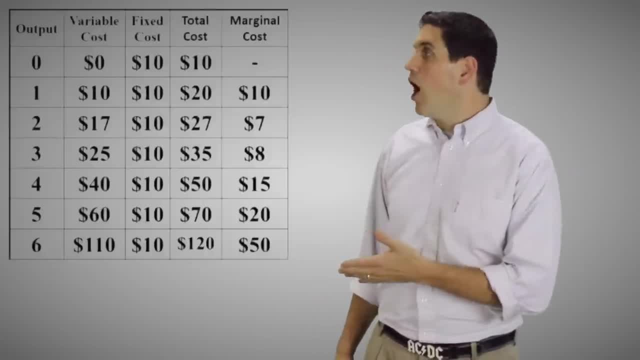 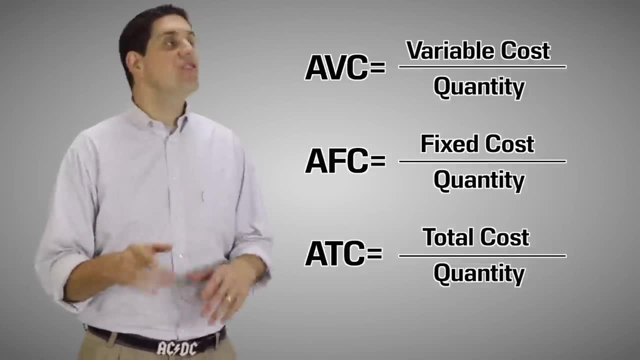 So the average variable cost is $10,, $15,, $20, and $50.. Now that you can calculate these costs, let's calculate the per unit cost. There's average variable cost, average fixed cost and average total cost. The average variable cost is the total variable cost divided by the quantity. 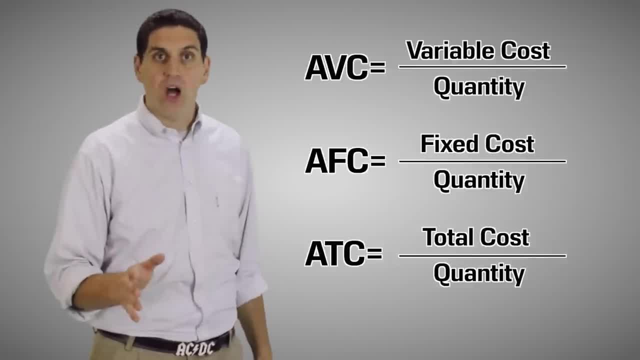 Average fixed cost is the fixed cost divided by the quantity, And the average total cost is the total cost divided by the quantity. Most of the time when you see these, you're going to see them by the acronym, So AVC, AFC and ATC- Get used to that. Now let's go see if you can actually use. 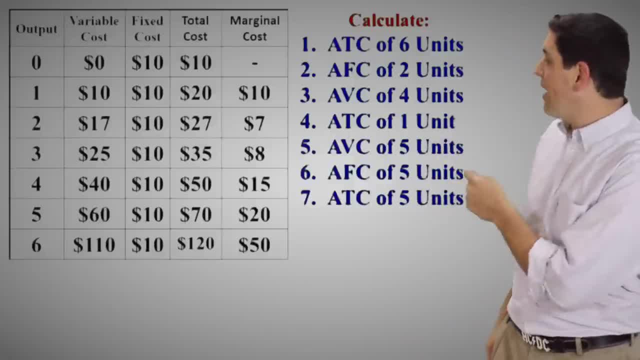 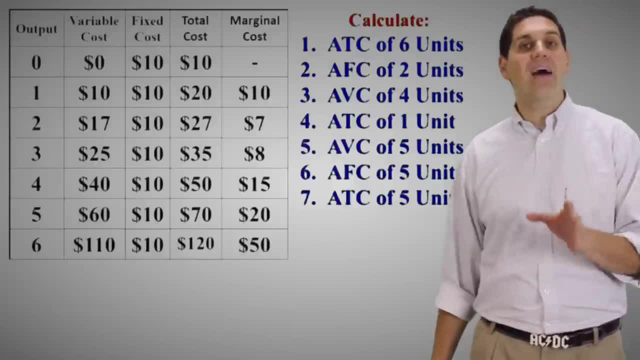 those equations and calculate the average cost curve. I want you to calculate the average cost curve: Average total cost of six units, The average fixed cost of two units, The average variable cost of four units, The average total cost of one unit, And calculate all three. The average variable. 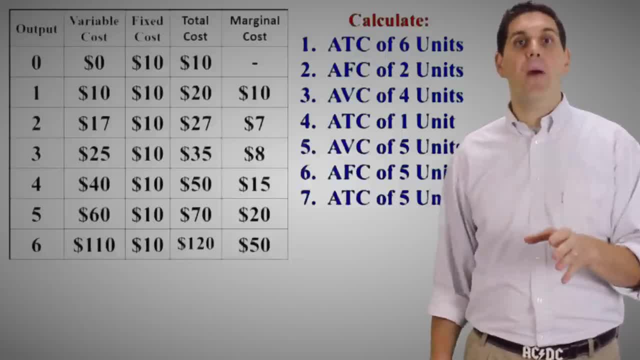 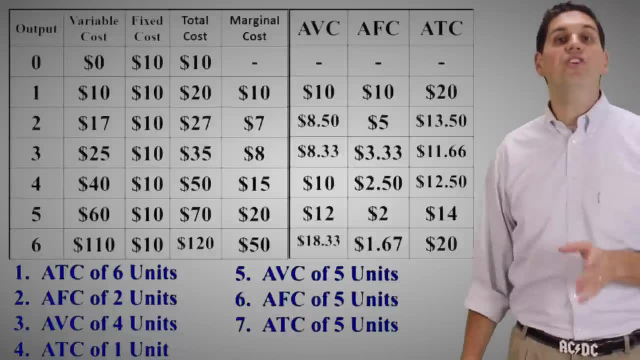 average fixed and average total for five units. So go back to your paper, number one through seven, and make sure to calculate each one of these. Pause the video and I'll go over them. All right, the average total cost of six units is $20.. That's because the total cost is $120,. 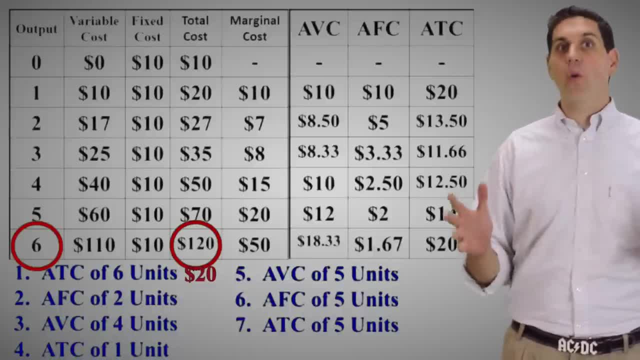 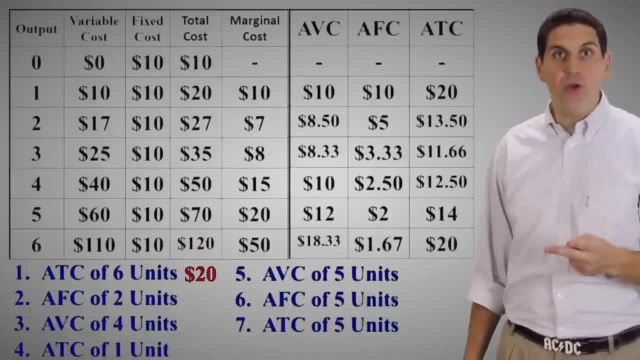 and we're producing six units. So if the total cost is $120, and you produce six units, how much did each one cost on average? Well, $20.. The average fixed cost of two units is $5, right, It's the $10 fixed cost divided by two units That gives us $5. 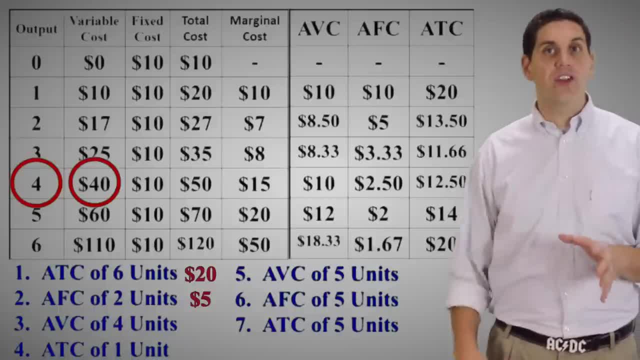 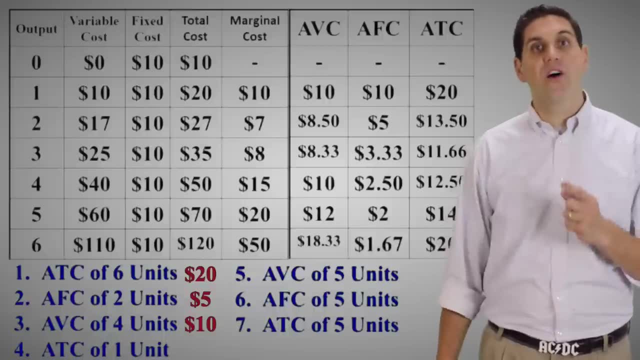 The average variable cost of four units is the $40 variable cost- total variable cost- divided by the four units that we produced. So it's going to be $10.. The average total cost of one unit is $20.. If one unit costs a total of $20, then on average, 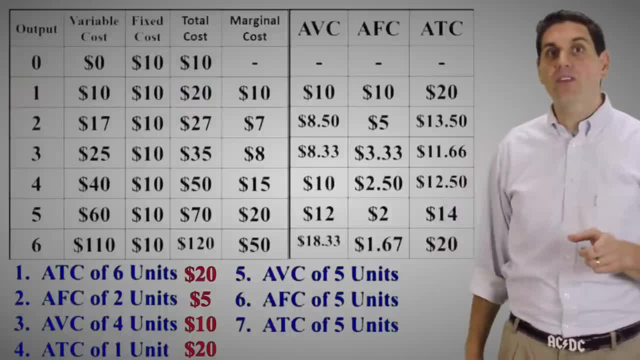 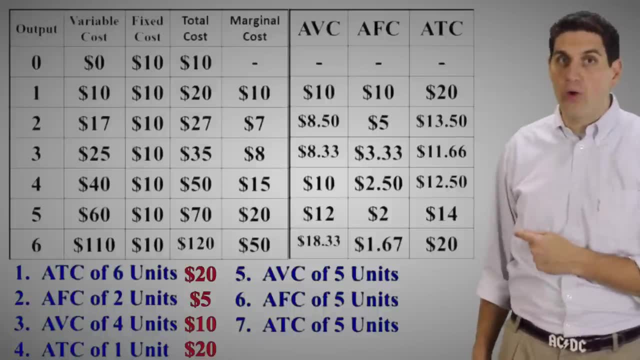 that one unit costs $20.. Now let's take a step back and find out something you might not have noticed first time around. Notice that the average variable cost plus the average fixed cost equals the average total cost. For example, for five units, the average variable cost was $12,. 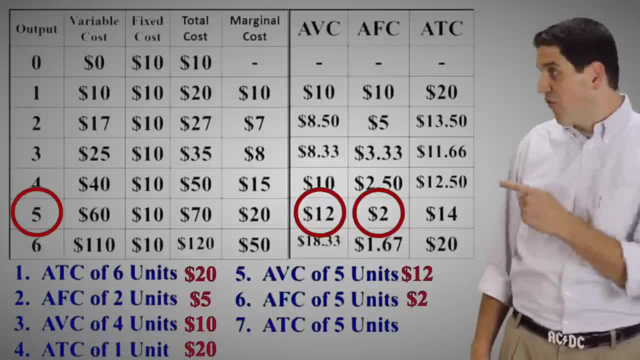 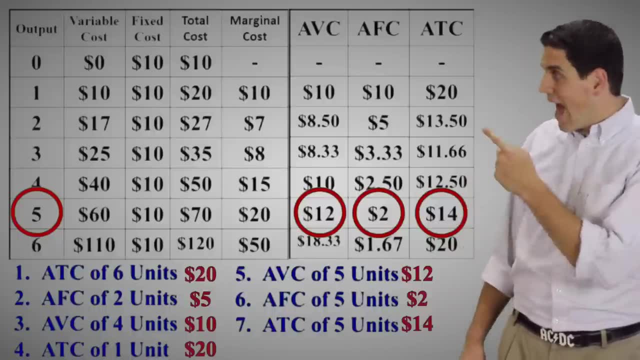 the average fixed cost was $2, and the average total cost was $14.. 12 plus 2 equals 14.. That's how it is. for every single one of these, The average variable cost plus the average fixed cost equals the average total cost. Actually, it is not that bad. 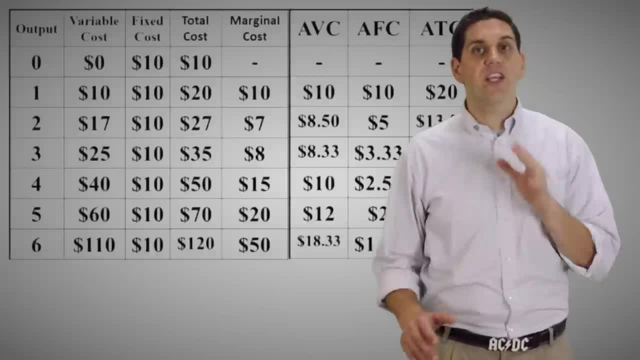 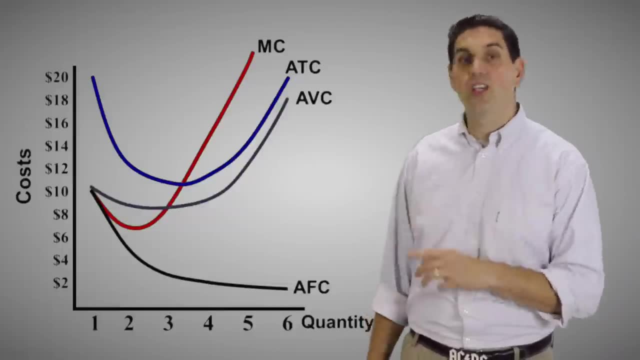 I kind of like cost curves. The next thing you're going to do is you're going to take all these costs from the chart and you're going to put it on a graph. To learn more about that graph and to find out how to use it, you've got to watch the next video If you like these videos.